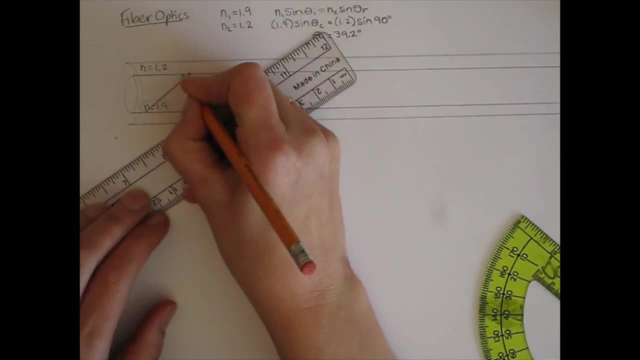 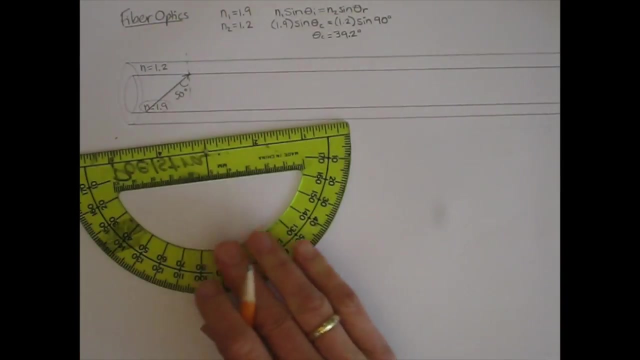 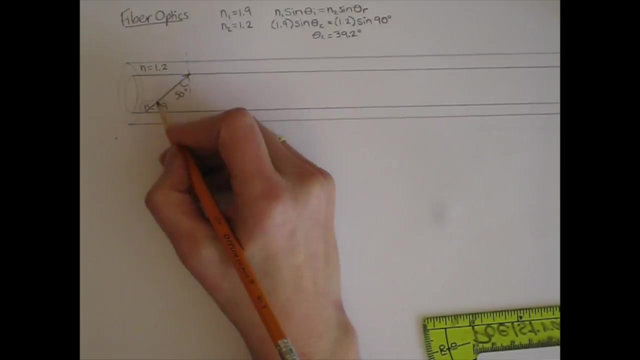 But I'm starting inside, inside the core. Okay, So my incident angle is 50 degrees and I want to double check that that is right, 50 degrees. Okay, So my light ray is incident in this higher index of refraction. 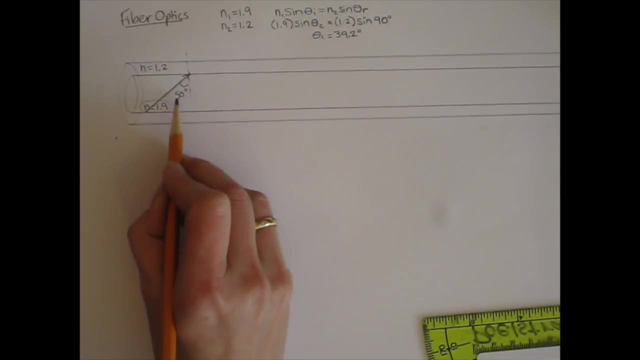 Okay, So I'm going to measure the higher index of refraction material at 50 degrees. When it hits this boundary- because 50 degrees is bigger than the critical angle- it will have total internal reflection. Well, reflected angle is equal to the incident angle. 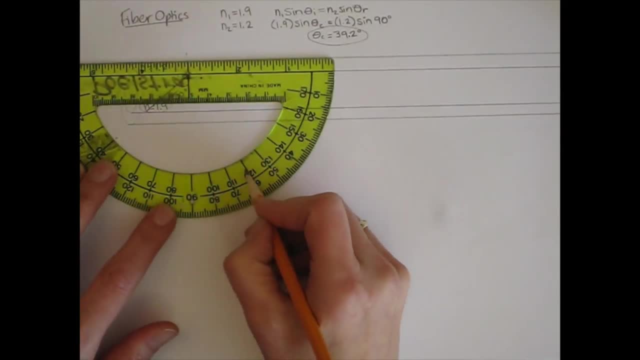 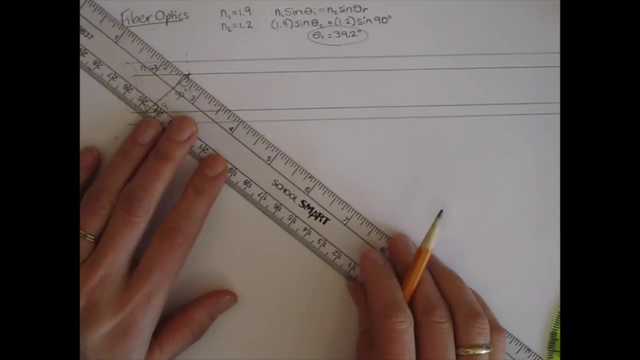 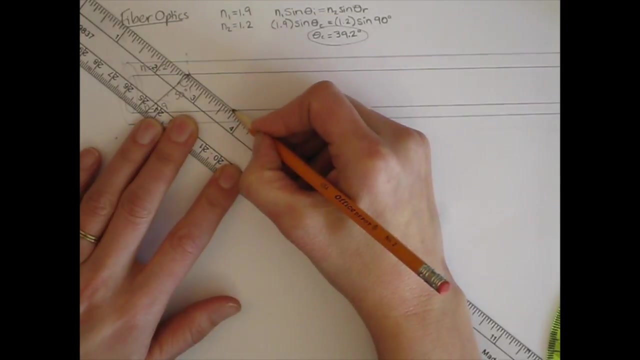 So I just need to measure 50 degrees from the normal 10,, 20,, 30,, 40,, 50.. So here's the light ray bouncing now off, reflecting off that boundary. Okay, Now don't get carried away when you're drawing this light ray, because right here now it's. 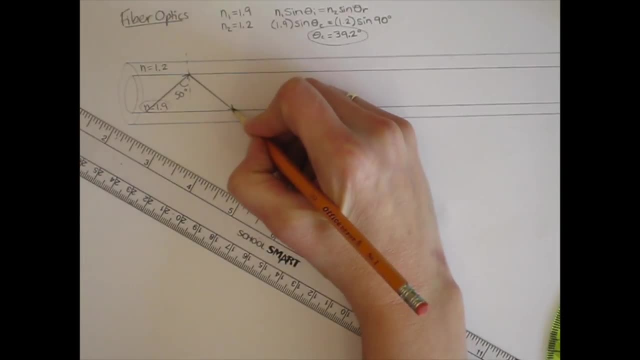 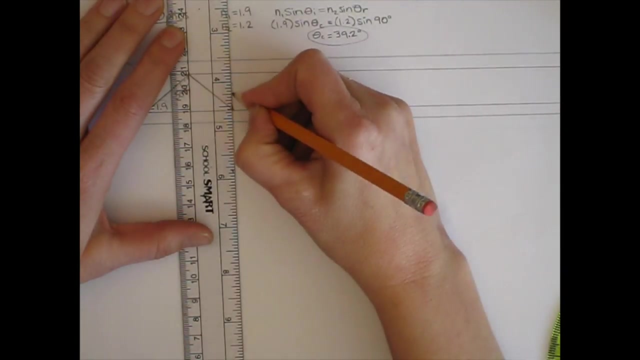 hitting a boundary, It goes in a straight line until it hits another boundary. Then you have to figure out what's going to happen now. Is it going to refract through this boundary? This is a boundary between the 1.9 and the 1.2 material. again, 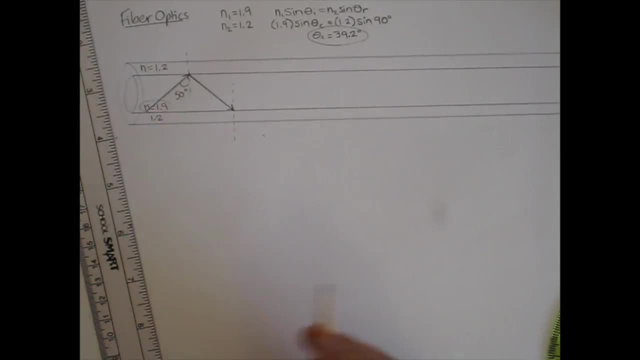 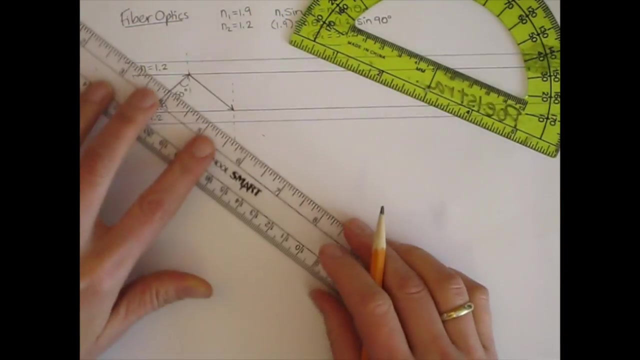 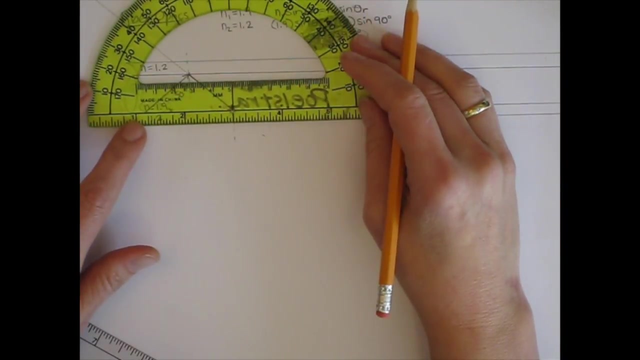 Remember the 1.2 material surrounding the core. Well, what is the angle of incidence? Okay, You can measure it, or you could use geometry, but if you measure it, you're probably going to need to extend your light rays so you can measure them with a protractor this large. 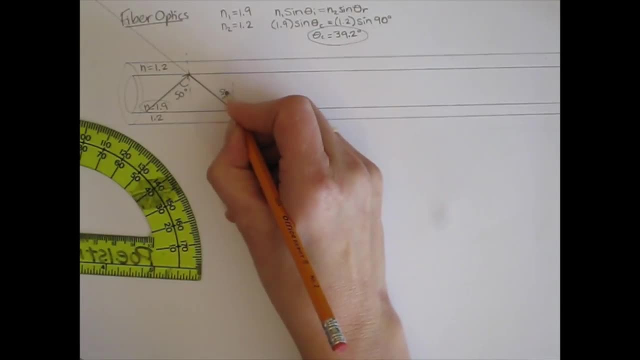 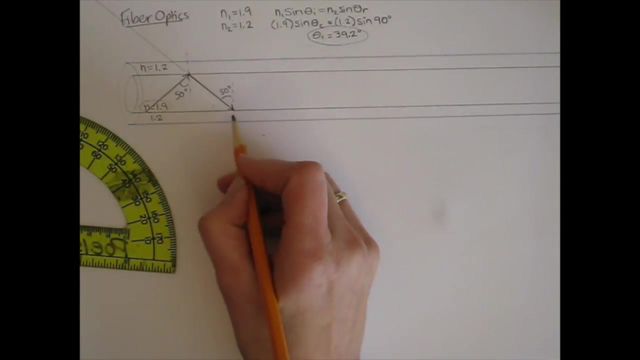 So it looks like 50 degrees. Well, what's the critical angle for this boundary? Well, it's incident in the 1.9 material and it's going to the 1.2 material, So it's the same exact boundary that we saw. 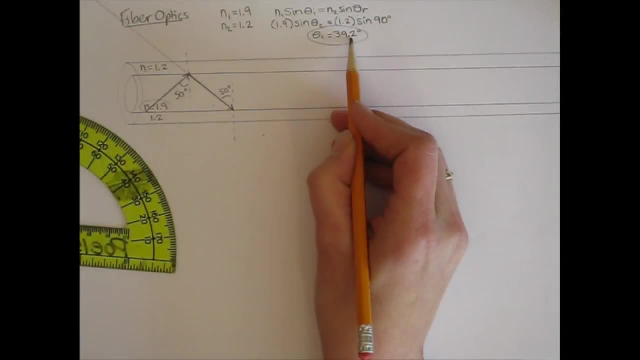 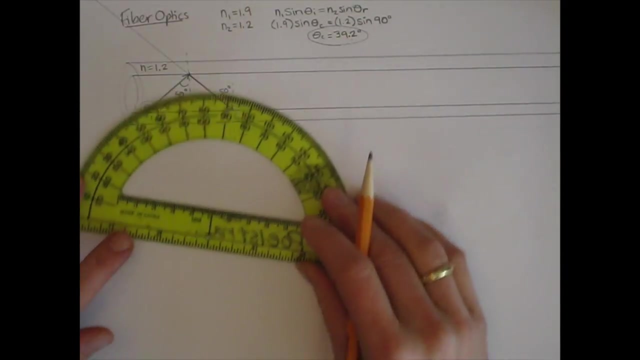 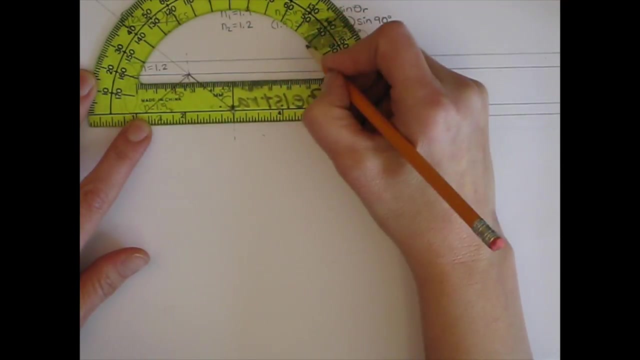 It's the same exact angle that we had at the top of the core, So the critical angle is still 39.2.. And since our incident angle is larger than 39.2, we have total internal reflection occurring again at 50 degrees.